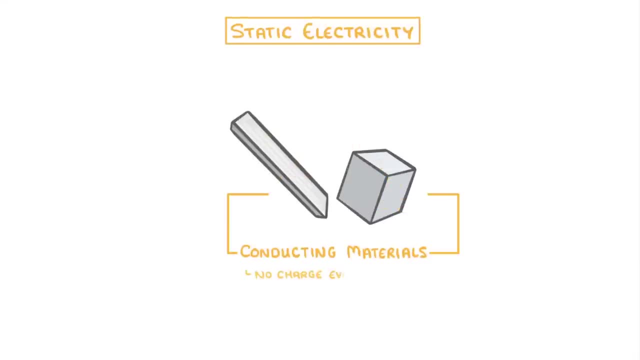 just flow straight back again, and so no charge ever builds up. In insulating materials, though, like a polythene rod and a cloth, the electrons can't flow back, and so the transfer caused by the friction gives a positive static charge on the material. 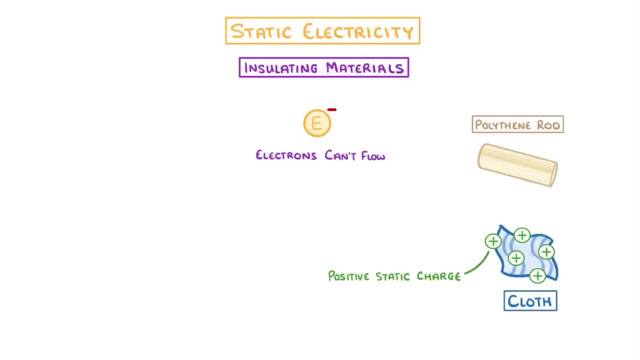 that lost the electrons- in this case the cloth, and a negative static charge on the one that gained them, the polythene rod. Which way the electrons get transferred each time depends on the specific materials involved. For example, if we took a similar cloth and used it to rub an acetate rod instead, then the electrons 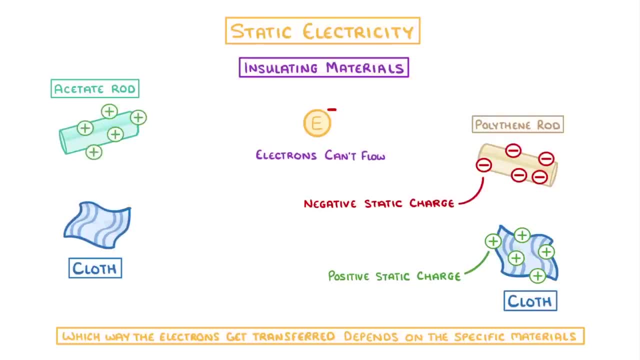 would get rubbed off the acetate rod, leaving it positive, and onto the cloth, making it negative. In any case, the key point to remember is that it's only the negative electrons that are transferred. The positive static charges occur because an object has lost negative charge and not 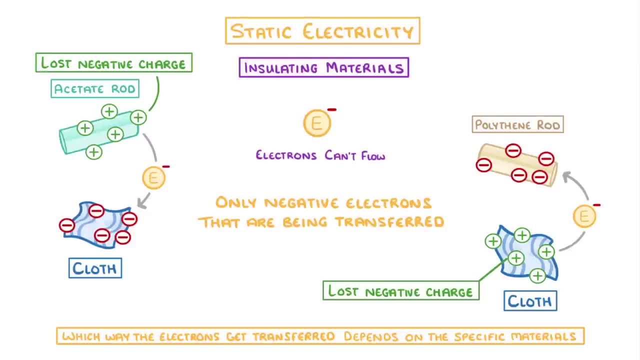 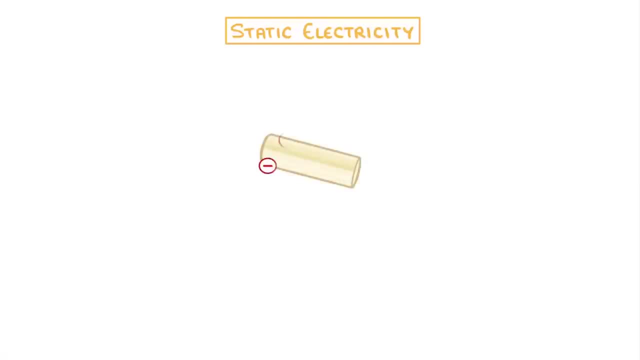 because it's gained positive protons. The next thing we need to look at is what happens if an object keeps on gaining negative electrons. As more and more electrons are transferred and the size of the charge increases, a potential difference will develop between the charged material and the earth or any earthed object. 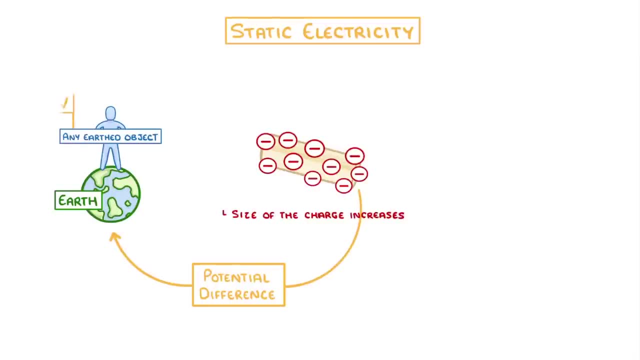 like us Because, remember, earthed objects are always at zero volts. If the potential difference between the charged object and the earthed object is large enough, then electrons can jump across the gap, And that jumping of electrons is what a spark is. 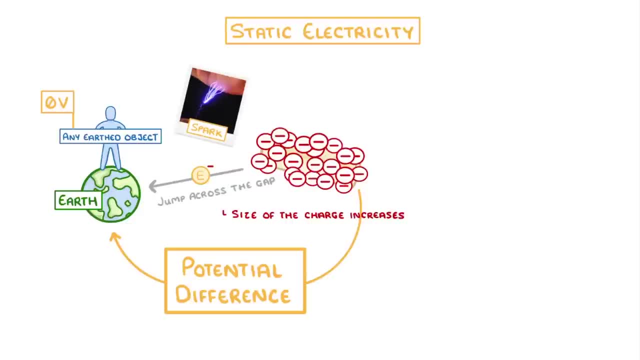 One thing we need to point out is that charges can sometimes build up on conductors too. It's just much less common. For example, cars can build up charge because their metal frame is in contact with the wind, which can transfer electrons. 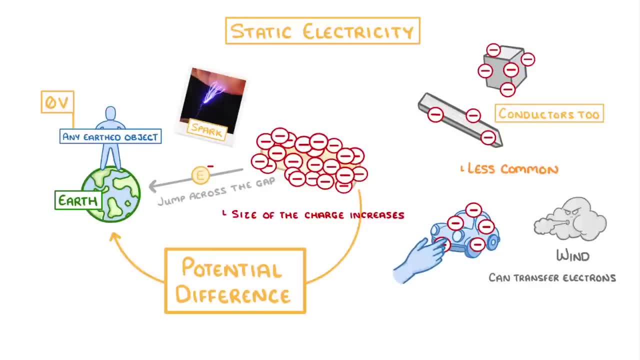 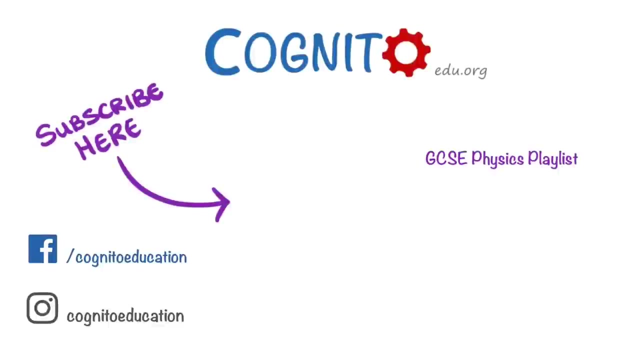 You've probably experienced this yourself when you've touched a car and got an electric shock. This is just a small spark from the car discharging to the earth through your body. Anyway, that's everything for this video, So if you enjoyed it, then do give us a like and subscribe, and we'll see you next time.